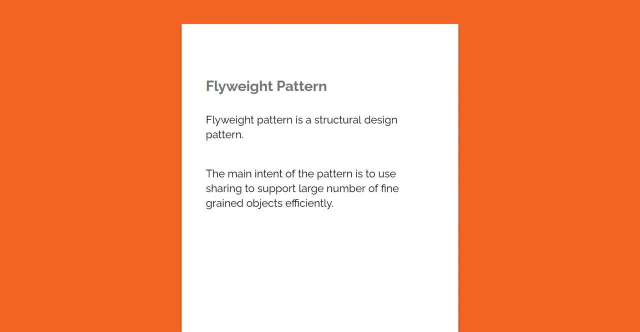 Now, if you are just creating an object five times or six times, I think it's an overkill to use this design pattern, but imagine a scenario where you are creating hundreds of the same object again and again, and again. this is where this design pattern will be extremely handy. So for today's discussion, we are going to talk about a scenario, and let's 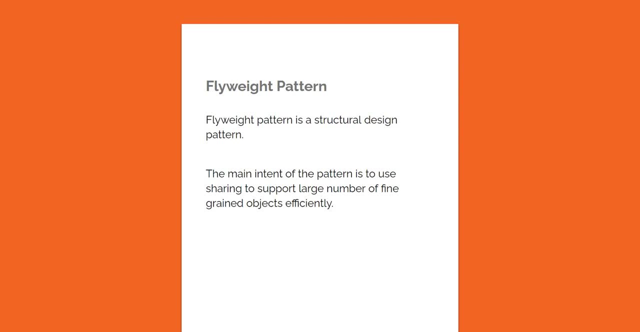 say, there is an application which is used for showing the location of car, and consider that this application is a distributed application and it keeps all the car's information in memory on some sort of server, and if that application is served to hundreds or thousands of user, creating. 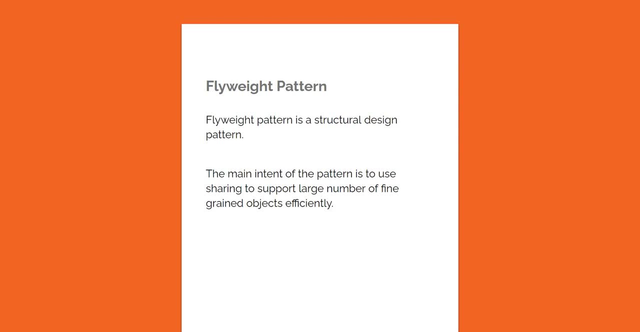 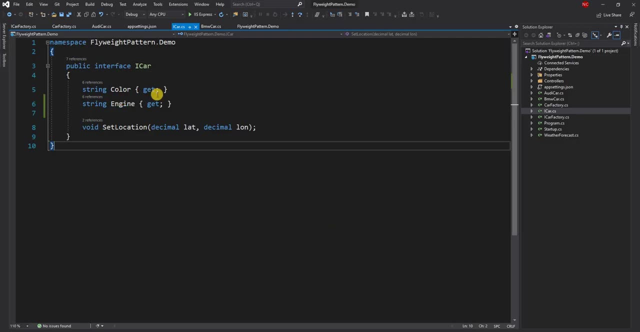 a car object every single time will take a lot of memory, and that is the case where flyweight design pattern will come in handy. Let's open the C sharp code and let's say this is the interface which we are going to be dealing with. We have a car which has two properties: color and engine. 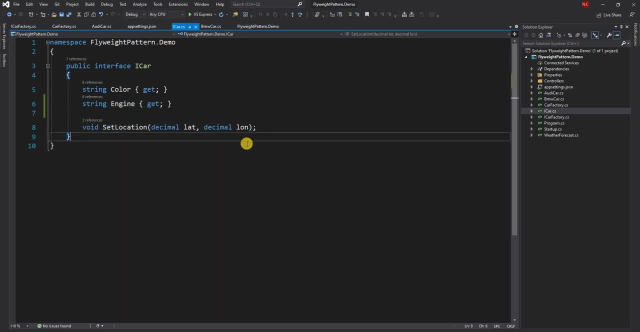 and then there's a set location which is used to set the location of the car, meaning where the car is right now in a map. There are two different states of this object. first state is kind of a static state which is the color in engine and once it is set it is not going to change. 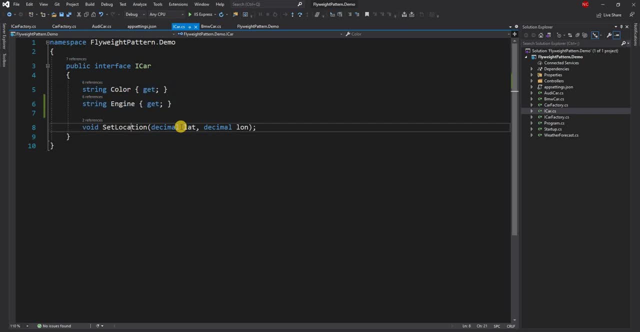 throughout the lifetime of a particular object, whereas the location, which is the latitude and longitude where the car is currently, is going to change based on the context, based on where the car is right now. So, when you design flyweight design pattern, this is where we have to segregate intrinsic data, which is the information that does not change based on a context. 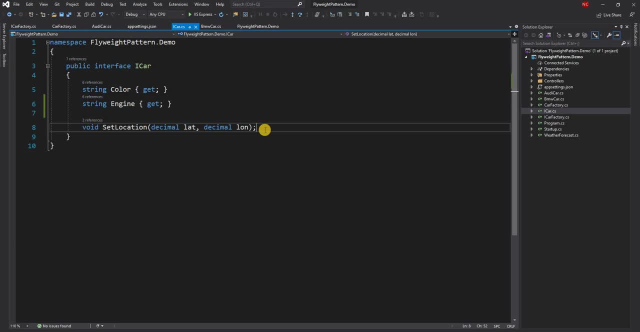 and the extrinsic data, which is the information which changes based on context, and in flyweight design, the class or the interface which saves the in-centric data is what is called as flyweight, and in our case it is the class which will derive from icur is what the flyweight is, and then we'll create. 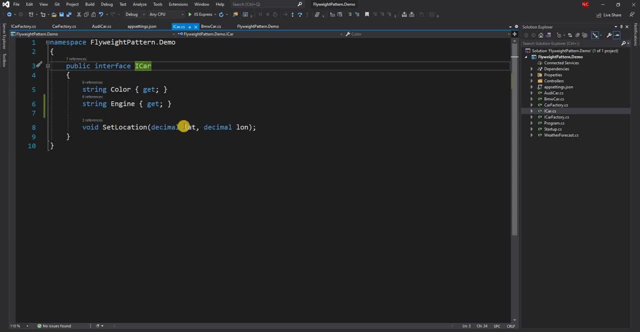 a contextual object which will be responsible for saving this contextual state of the object, which is lat and long. Now one other thing to keep in mind: if your class just has like two or three properties, which means it's anyway very lightweight, again flyweight might be an overkill. 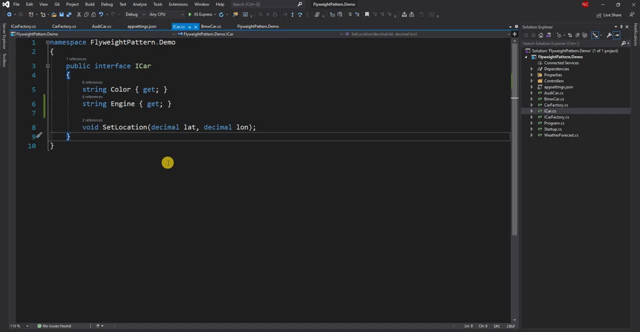 It should be used only in case of objects which are heavy and they are expensive both in terms of memory and CPU during creation. So in this case, I kept it simple just for the simplicity of the example, but this is something to keep in mind when you use this particular design pattern. 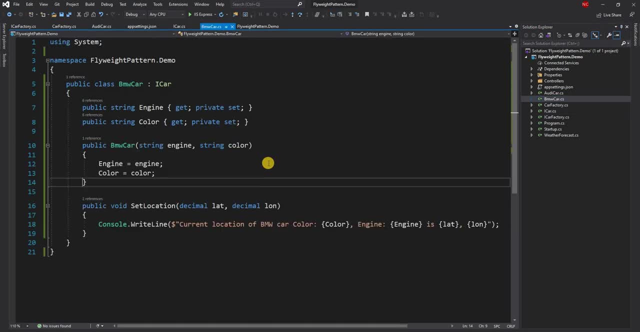 Now, in this case we have icur, and from icur I created two classes. one is a bmw car which implements these interfaces, which are set as a part of the constructor, and then set location, just prints out the location along with the car and the engine for the bmw car. Similarly, we have 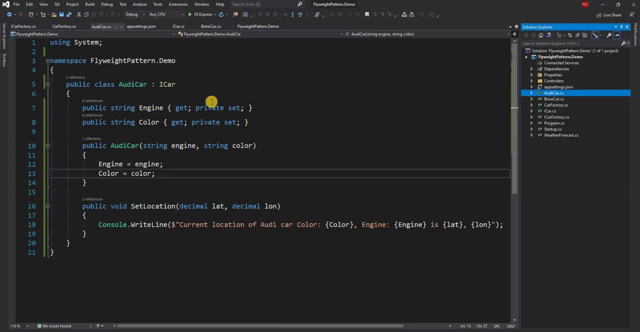 an audi car, which is very similar. So in this case, as you can see just from these two classes, the idea here is: all the bmw cars will share the same car object, instead of creating a new bmw car every time when someone has a bmw car and they want to see where their car is, Whereas the lat and long of the car is. 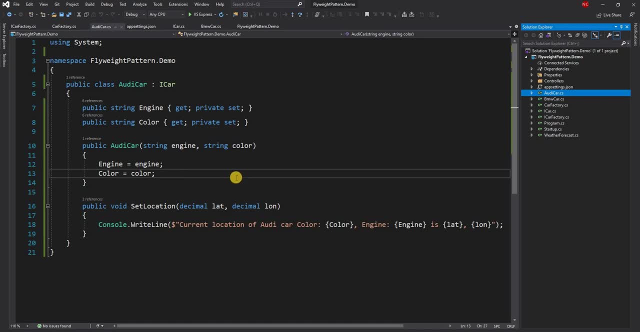 something which will be managed outside, and that is what will change for every single consumer of this application. So these are the flyweight objects, and how do we ensure that there is only one instance of each of this class? Well, there are a couple of ways to do it: The 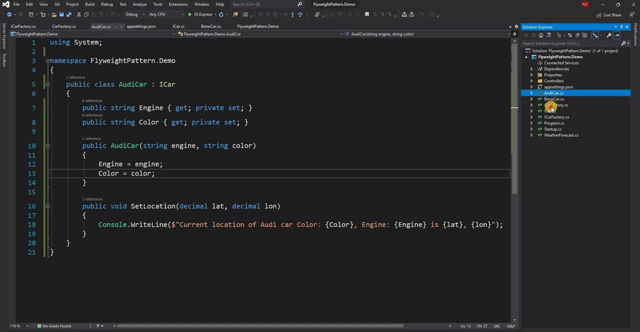 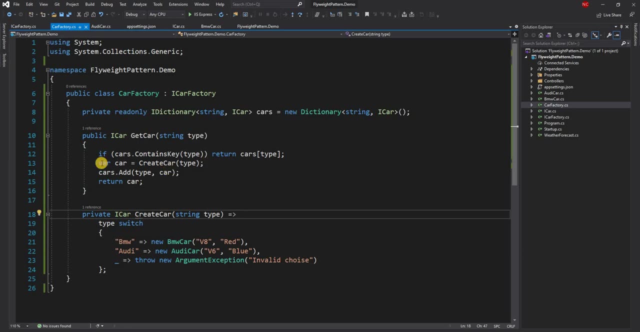 traditional way of doing it is through a factory. So here I created a icur factory. In the icur factory I have a dictionary which has a car and when someone calls get car, it checks if the car exists in this dictionary, then returns. If not, it just creates a car and then adds it to the 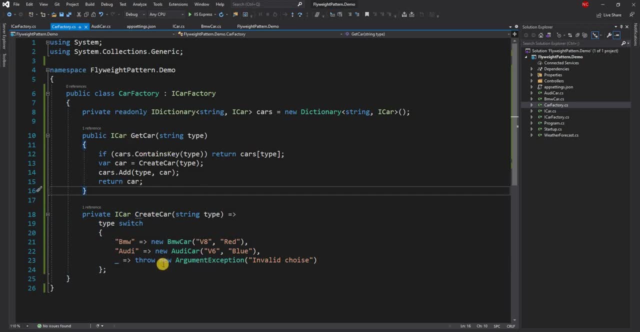 dictionary and then returns. As simple as that. This will ensure that a type of car is created only once, And here we are going to keep the car factory as a singleton class, So that there is only one instance of this particular class. So this is the factory. 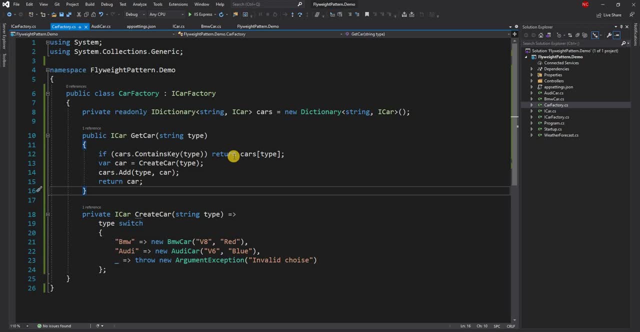 which will be used to create the car, to ensure there is one single instance, And then, finally, we need some sort of manager for the car which is going to manage the car itself and maintain the extrinsic data, or the contextual data, in our case, which is going to be latitude and longitude. 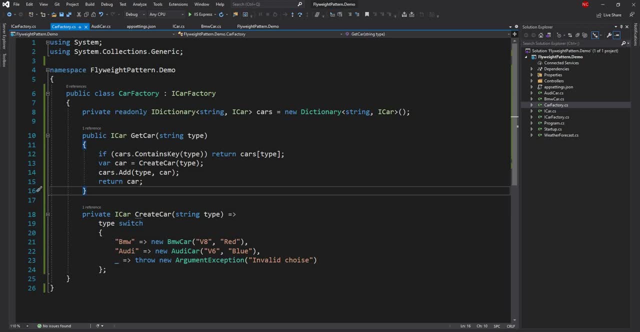 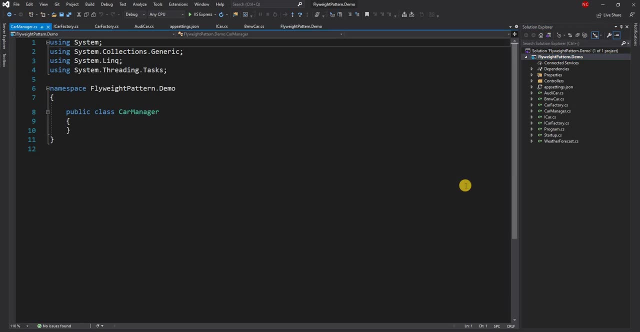 So for that what we can do is we can create a new class and we can call it something like the car manager. And here what we are going to have is the car manager is going to have a constructor And the constructor is going to take the type of the car, And then what we can do is we can 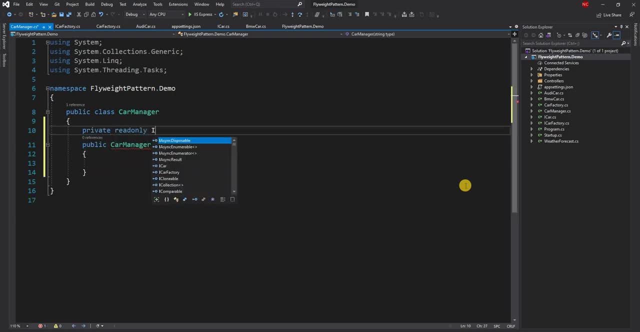 have a private read-only car car and we'll have car easy car And let's inject the I car factory also. Say: car factory dot, get car of type. That's about it. And then here, what we can also have is: you can have private. 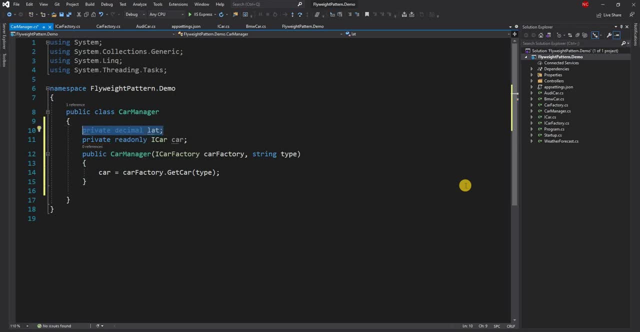 similar let and longitude, these two, and then we can have public void, set location, and here we are going to have longitude, and when this is called, all we are going to do is we are going to set the- and let's set these values- zero, a startup value, and here we can take the incoming values and select equal to that. 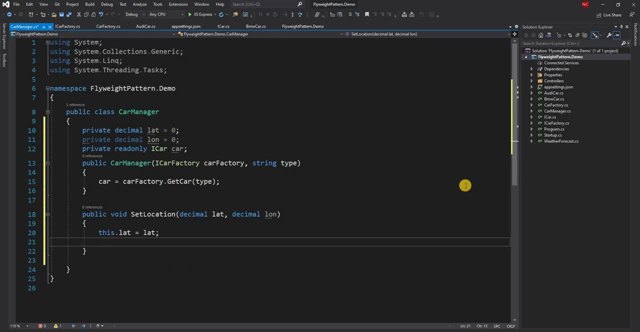 longitude, and then what we can do is we can say car dot, set location and then we can pass the location. so as you can see, here this class essentially is the class which is managing the contextual state. so every time a location is set, it is maintaining what is the current location, and then it is just 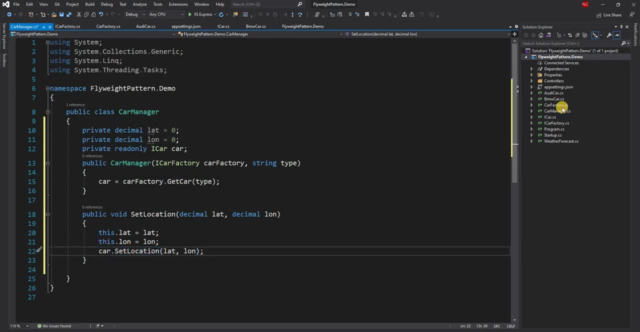 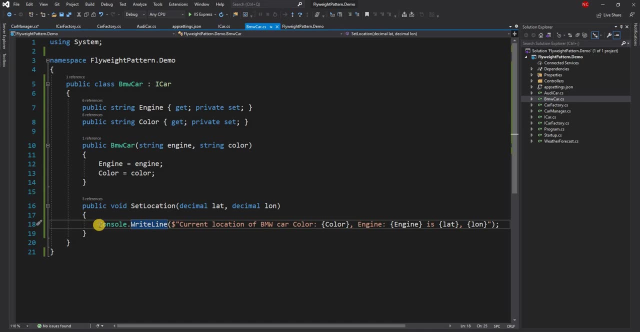 passing that location to the car to print it out. now, if you are dealing with a web-based application- and this is your server- when this set location happens you might be sending out a web socket message through signal or at this point in time, so we can say car dot set location and then we can. 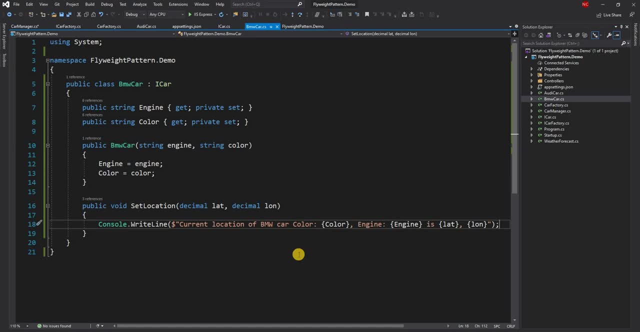 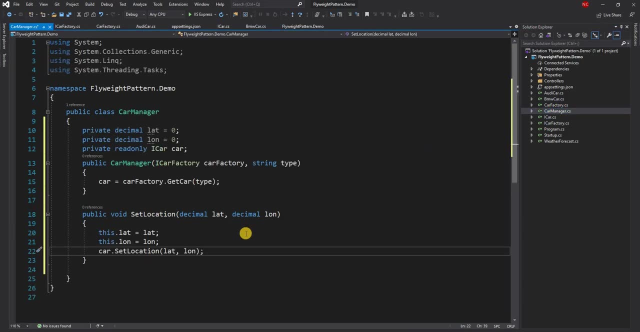 pass that location to the car so that the location of car is visible somewhere in the map. but for simplicity we are just printing it out here in console dot right line. so now the car manager, essentially, is going to set it up and consider the scenario where, if we did not had flyweight, 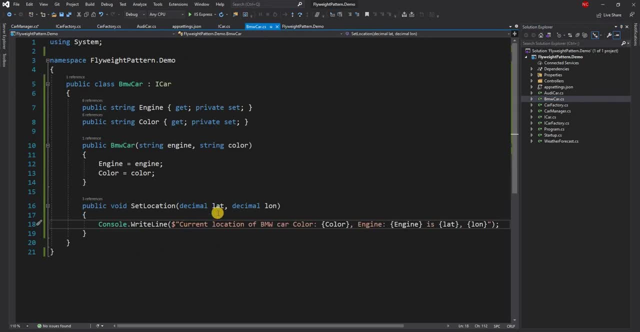 then all we are going to do is we are going to create the instance of bmw car like 500 times and here, as i mentioned here, it might not be a big deal because we just have two properties, but if we had 100 of properties it's going to take up a lot of memory, whereas for the car manager, given 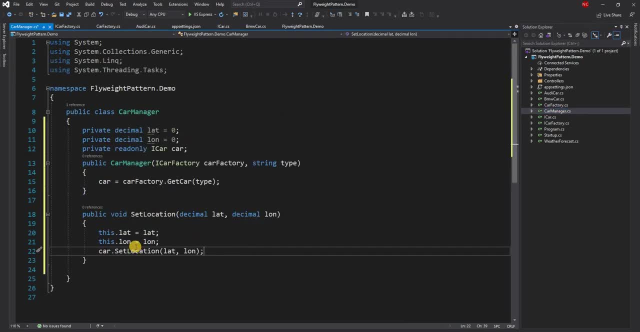 the car manager will be created multiple times. but since the car manager does not have anything except these two attributes, the actual size of the car manager will be minuscule compared to if you had to create it 100 cars. so that's where the advantage of flyweight design pattern comes in. 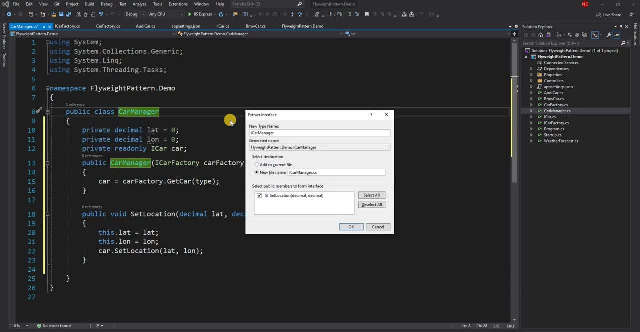 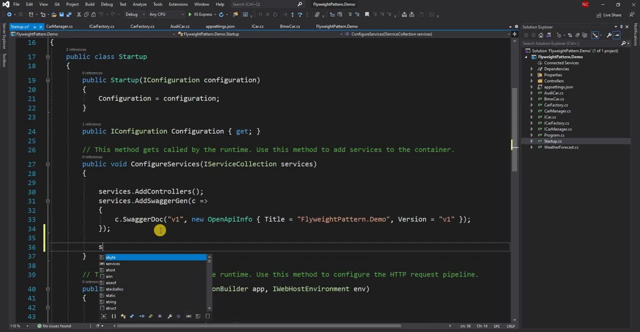 now that we have that, let's create an, let's create an interface for icar manager. and now let's go and in the startup. first let's add the services dot, add singleton, and we are going to add icar factory. car factory is the first one and, as you can see, the car factory is has to be a singleton class. 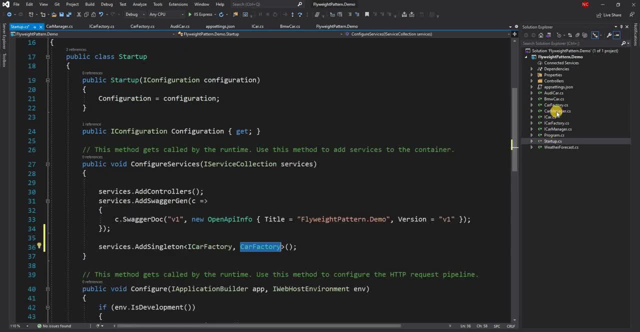 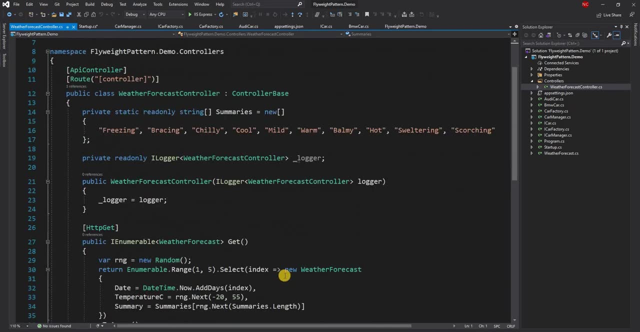 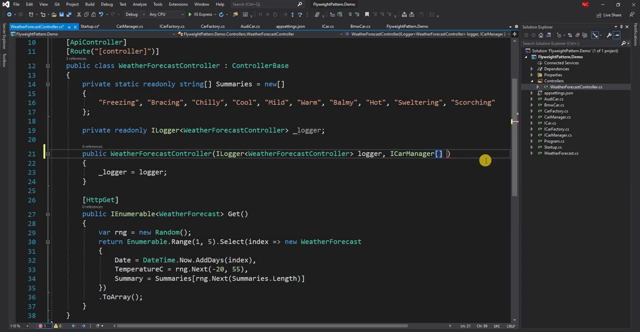 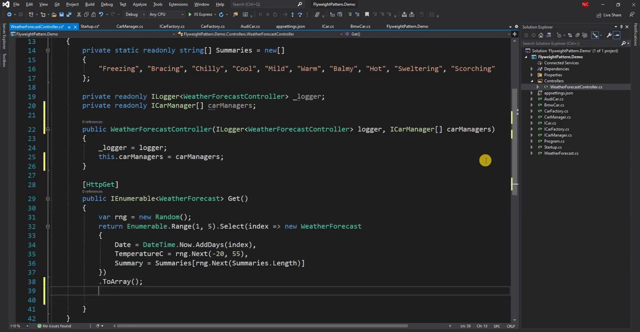 and then the next thing is: we want to use the car manager. now, let's use it in the controller. i'm going to use the default controller which comes in, instead of changing anything here, and here we can have i car manager, array, car managers- let's define this, and here we're going to call for. 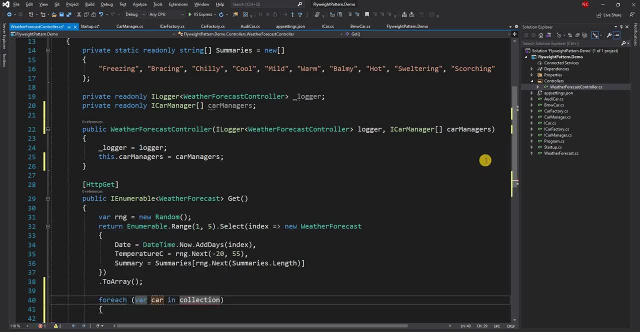 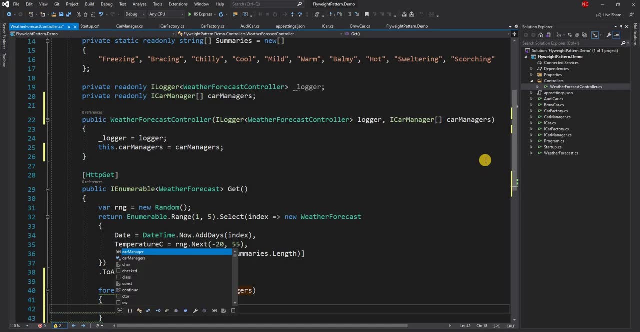 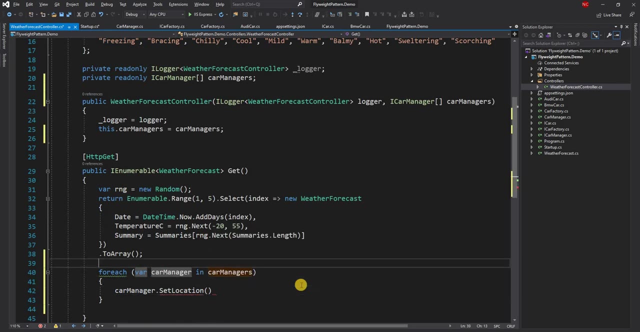 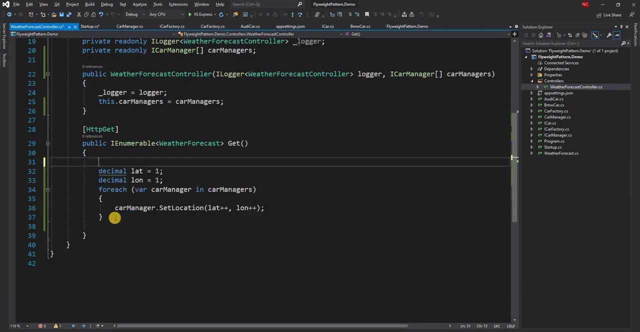 each, each car manager, car manager dot set location for lat long. let's do one thing. let's declare so we'll increment after every set and let's move this to the end. okay, so i'm keeping this. i don't want to change the implementation here, so that's all we are doing. 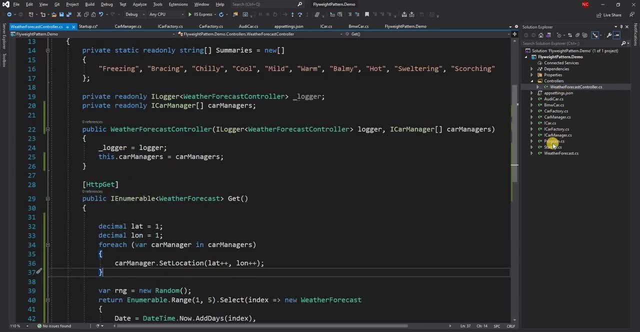 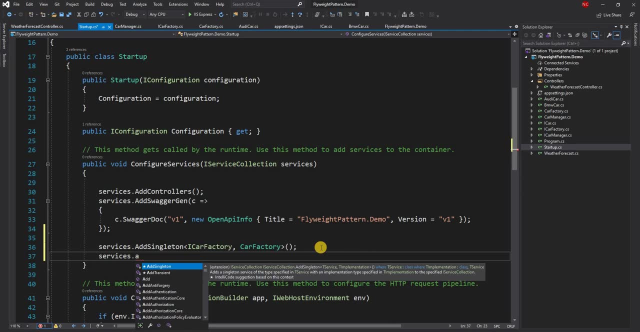 here we are setting the location. now it expects a car manager. so let's go into the startup and here what we can do is- and this can be also singleton, and this can be also singleton, and this can be also singleton, and this is an array, new car manager array. 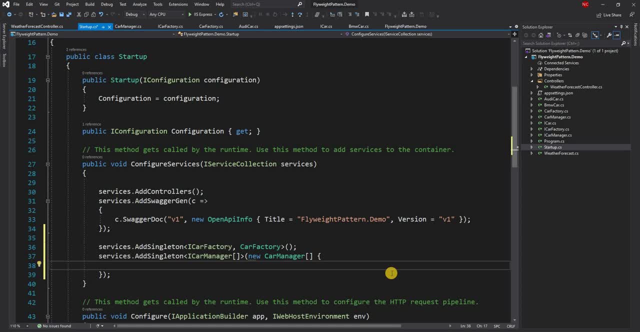 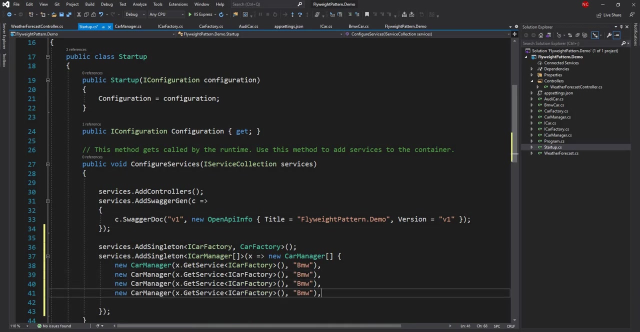 and here and here we can pass new car manager. the type is bmw comma, and here let's use this format so that we can do x dot, get service of i car factory, so it sends the car factory from the container. and then let's create a few of those. 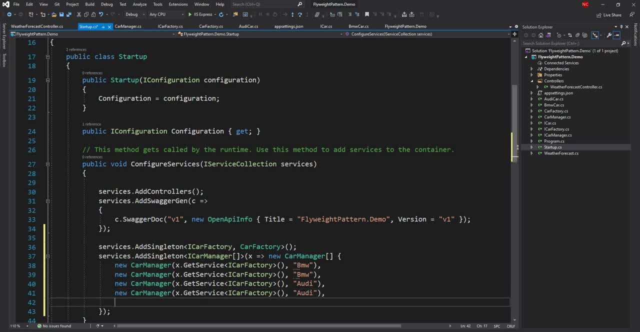 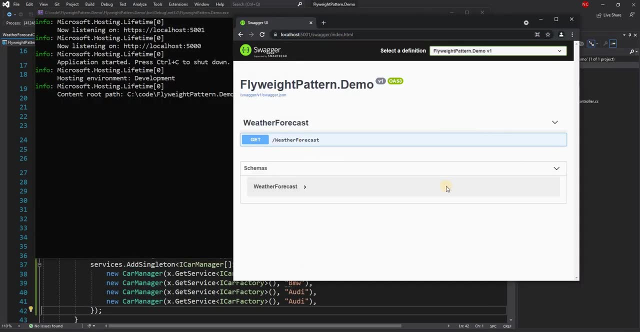 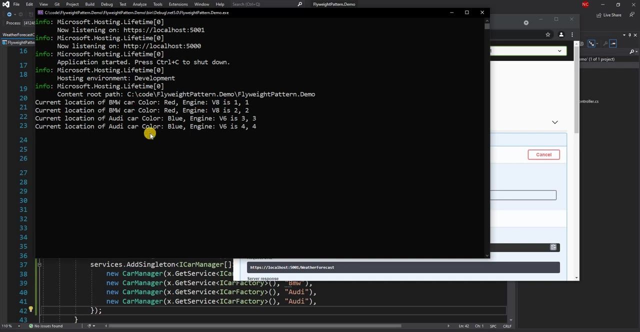 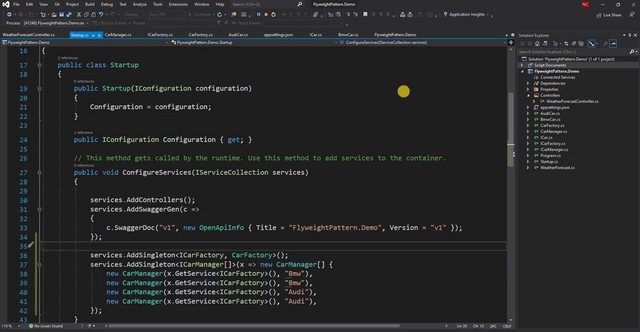 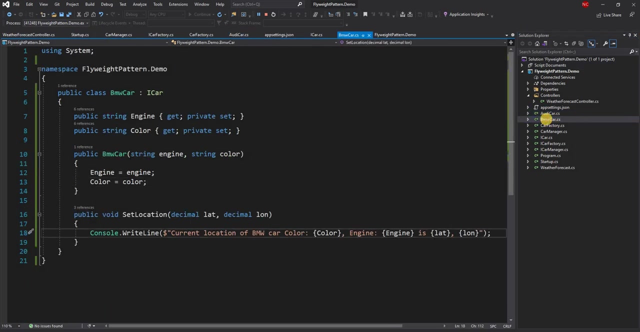 so couple of bmw, couple of audi and then, if we run this application now, now as you can see it printed out, couple of bmw and couple of audi. now here, as i mentioned, the example is pretty simple and straightforward but, as you can see, it shows the main concept of flyweight design pattern, where the audi car and the bmw car are.